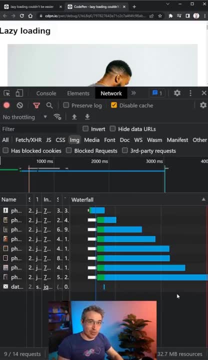 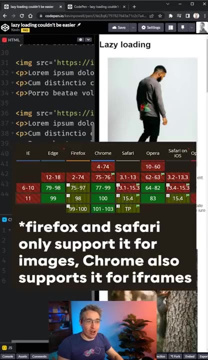 not scroll down or ever see those images, and they still are downloading them all. We used to have to use JavaScript with intersection observers or other things to bring in lazy loading, but it couldn't be easier anymore. All the browsers now support the loading equals lazy attribute, So you. 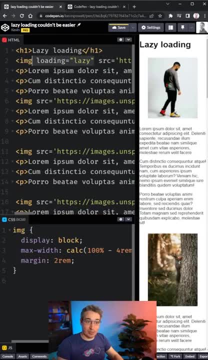 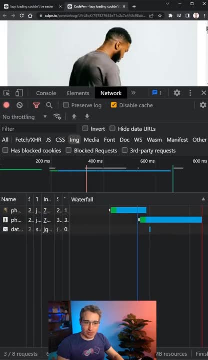 can just come on an image put loading is equal to lazy, So I'm just going to add this to all my images and we'll see the impact that this has. All right, so we're back on my page. Let's refresh and you'll see that only two images have actually loaded in. And as I scroll down the page, 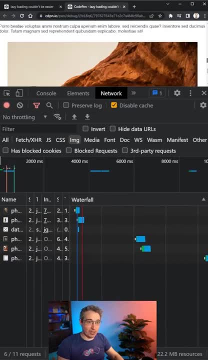 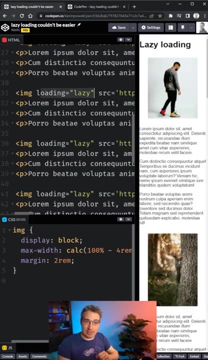 more images are coming as we go and the browser is deciding when to load them in, but it will do it before it enters the viewport and it does this all automatically. And so yeah, just a nice simple loading equals lazy, and you have lazy loading on your image. 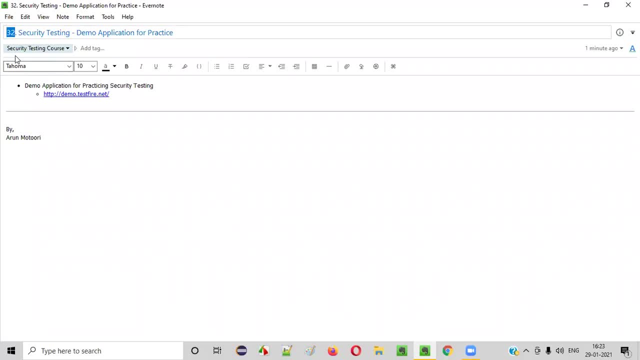 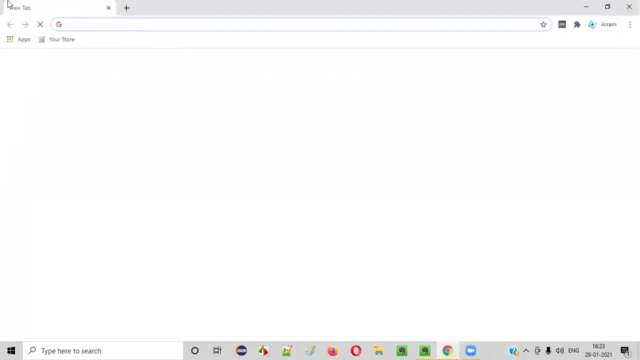 Hello everyone, welcome to session 32 of security testing video series. In this session, I am going to show you a demo application which you can use for practicing the security testing. So let's get started. Let's open any browser- guys say Chrome browser- and in that browser just type this URL of the demo application, that is demotestfirenet. 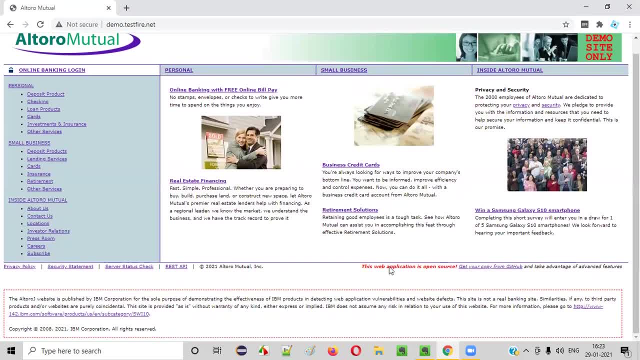 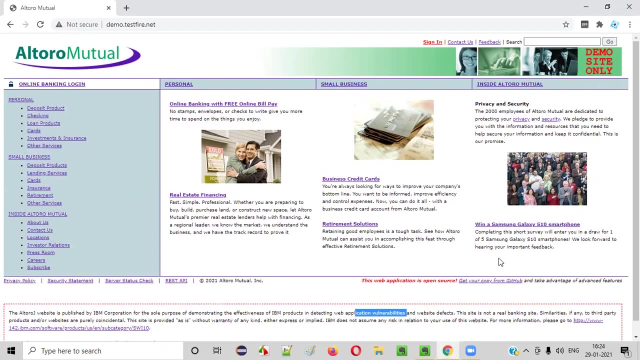 And you will be taken to an application, which is a demo application, where you can practice security testing by identifying different vulnerabilities. So, guys, this is a demo application, as I am mentioning, and as you already know, we should not be performing the security testing on some random applications. 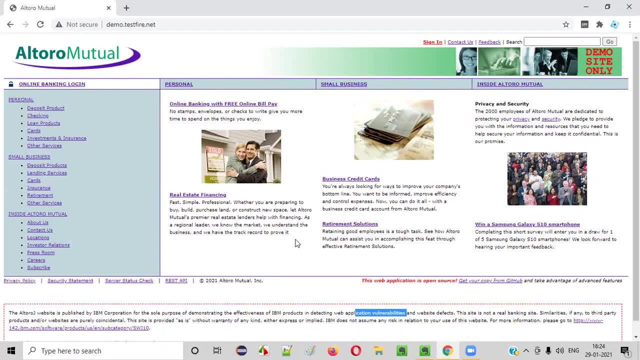 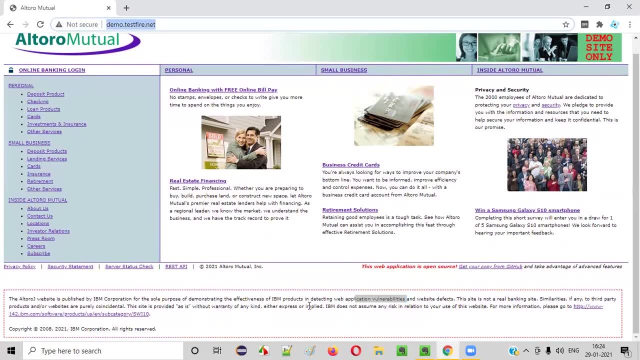 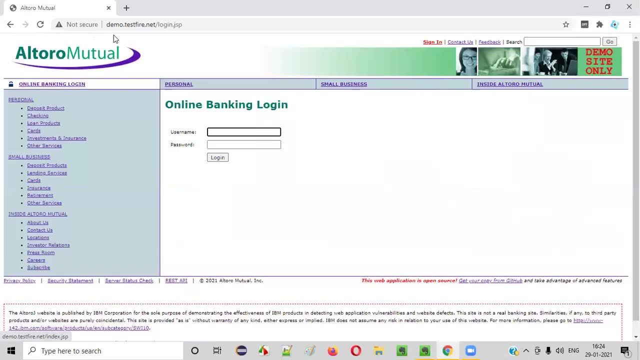 So you should only be performing the security testing on the application that you have permission for. But this application, that is demotestfirenet, is an open application. This is an open application where you can perform security testing and practice security testing. Let me navigate you through the sign in page of this website. Just click on the sign in option. you will be taken to the sign in page of this application.